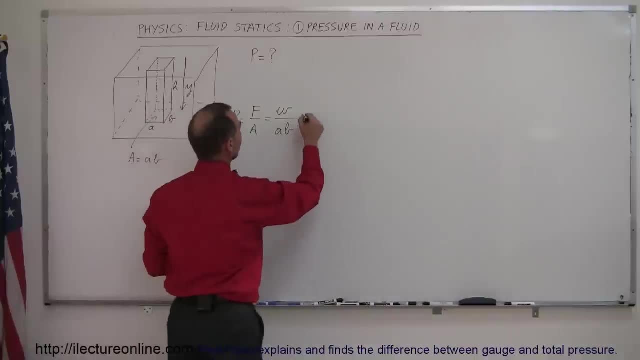 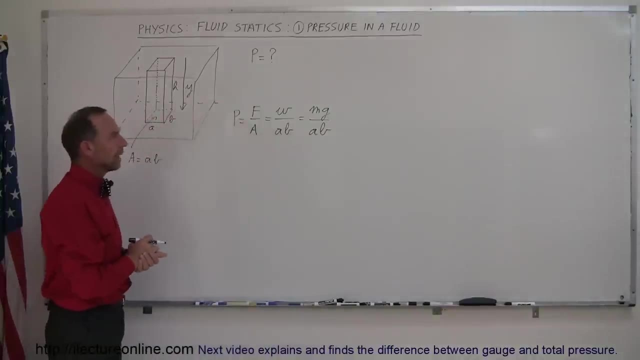 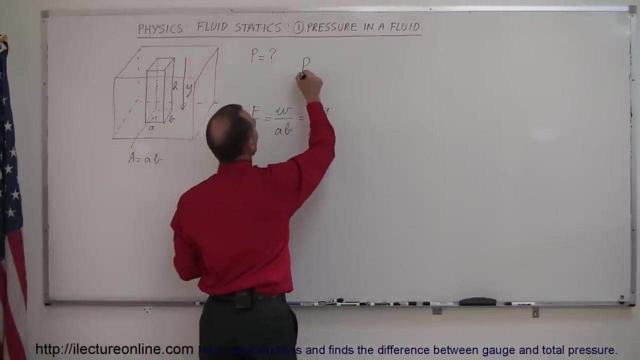 water is equal to the mass times the acceleration due to gravity. so this can be written as m? g divided by a times b. all right now, in fluids we have a relationship between the mass and the density, and that relationship is that the density of any fluid is equal to the mass divided by the. 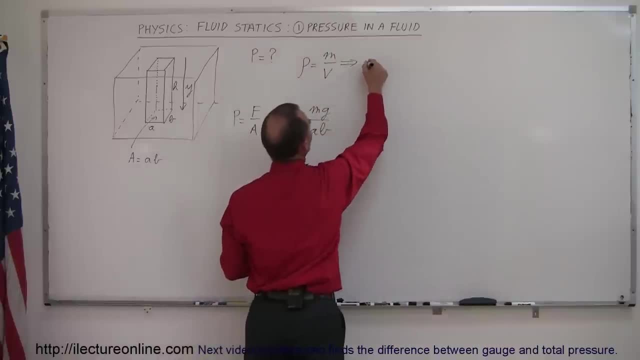 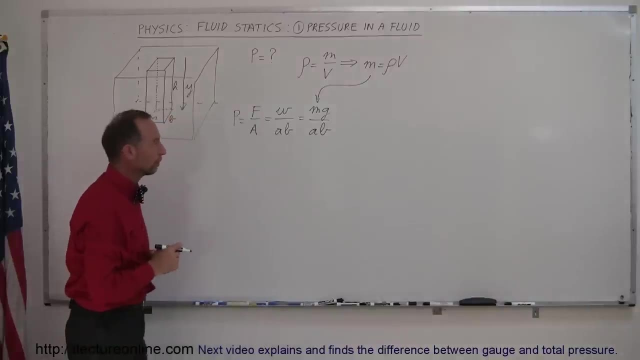 volume, which means that we can solve this equation for mass and write that the mass is equal to the density times the volume and substitute that in here for our equation for the pressure. so that means that now the pressure can be written as the density of the fluid and the mass can be written 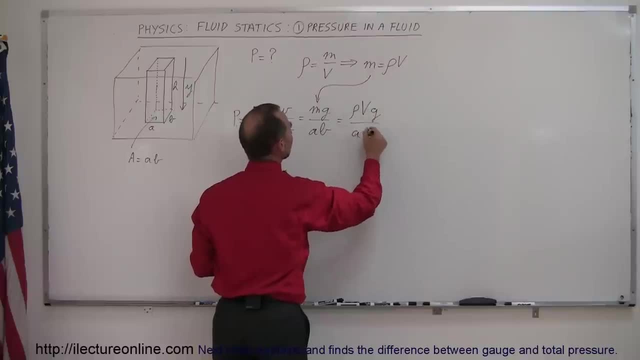 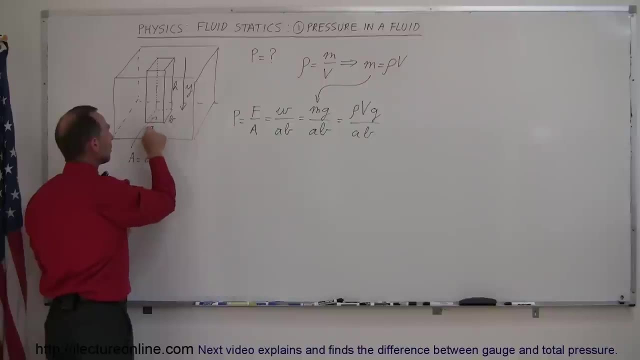 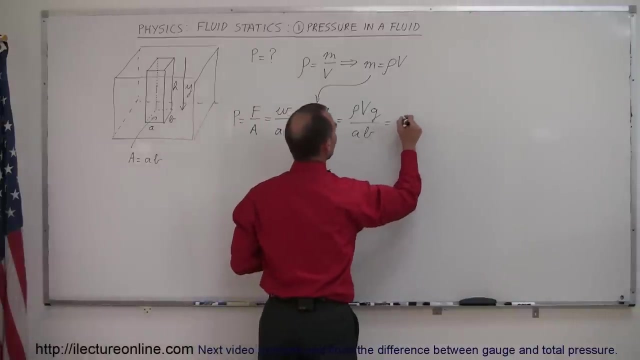 as the volume times g divided by a times b. excuse me, so the volume means the volume of this water column and the area underneath is simply still a times b and of course the volume of a cube is equal to this area of the base times the height. so this can be written as the density times the. 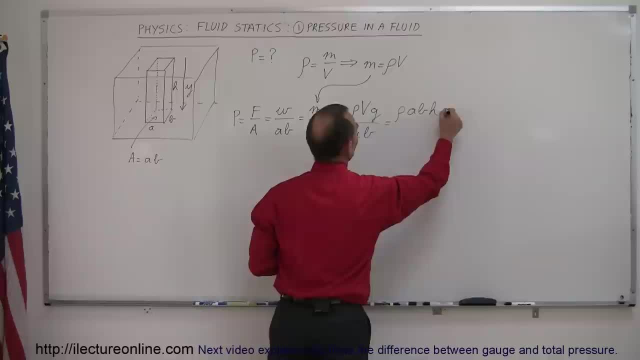 area of the base, which is a times b times the height, which is h times g. so volume is replaced by this. divide this by a times b and then, right away, of course, you can see that a and b are cancelled out. with other words, it's per unit area that gets cancelled out. and then, since the height, 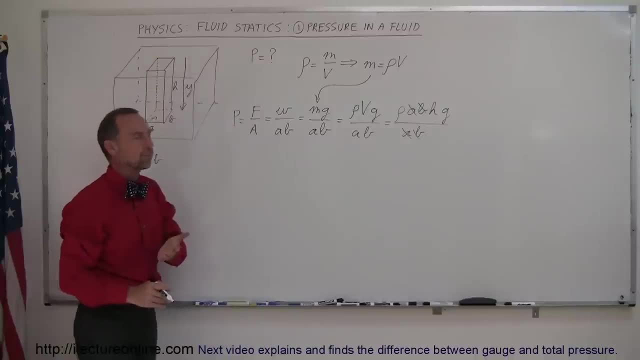 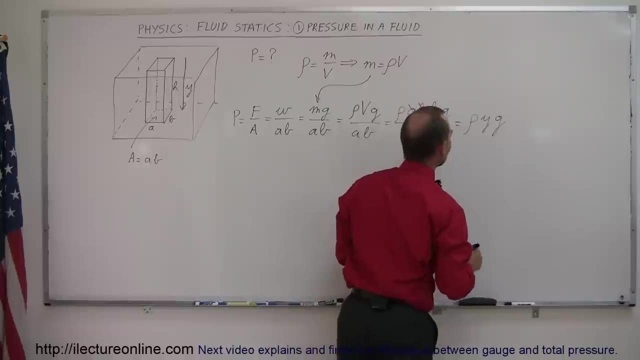 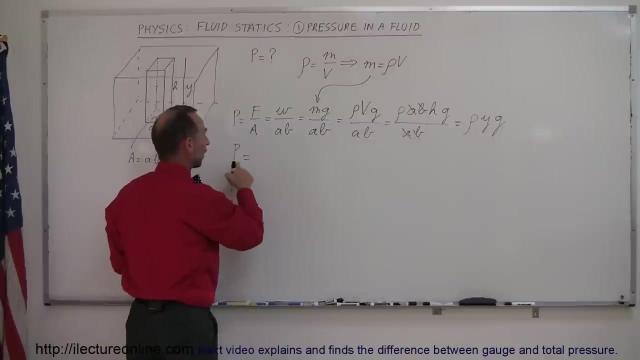 of the column is equal to the depth of the pool. we can then replace h by y, and so this can now be written as the density times y times g. and then, finally, the equation we like to use. we like to rearrange those terms and write it as the dense, the pressure at the bottom of the pool, which is 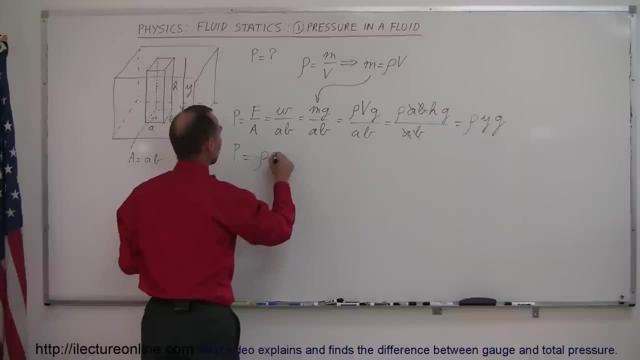 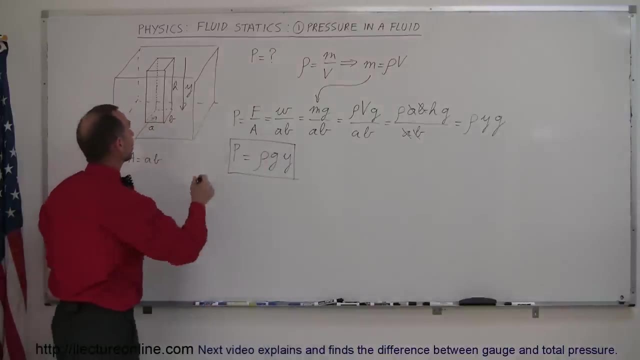 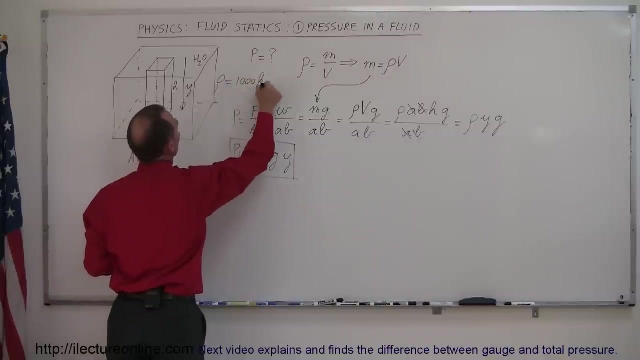 really the pressure at any depth. y can be written as rho g- y, and that's the equation we use to find the pressure inside the liquid. now, as an example, let's say that this is water and therefore the density is equal to 1000 kilograms per cubic meter. 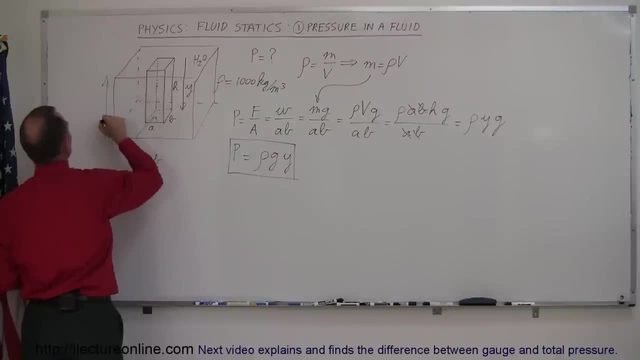 let's say that the pool is has a depth of 2.4 meters. that means that y is equal to 2.4 meters. and let's see what else do we need g? we know what g is. that's 9.8 meters per second square. 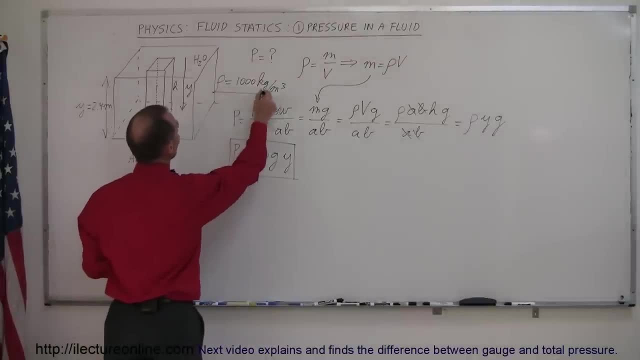 so in this case, the pressure, when we assume that the density is 1000 kilograms per cubic meter and the depth of the pool is 2.4 meters, that is equal to the density, 1000 kilograms per cubic meter, multiply times g, which is 9.8.